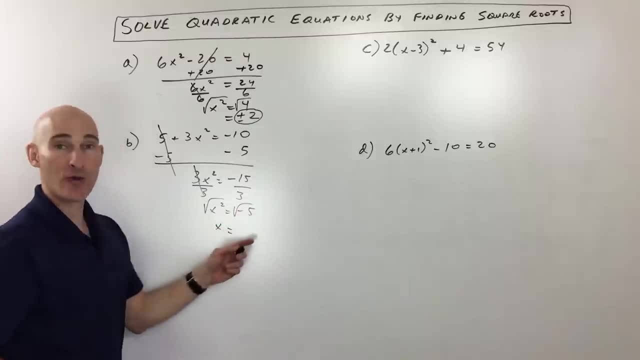 root, because that's the opposite of squaring both sides. Ah, but we have a problem here. We can't take the square root of a negative number. That's going to give us an imaginary number which you usually get into when you get into algebra two and pre-calculus. So for this one we're just going to 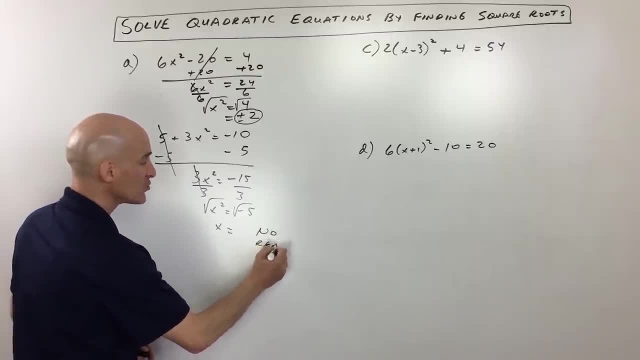 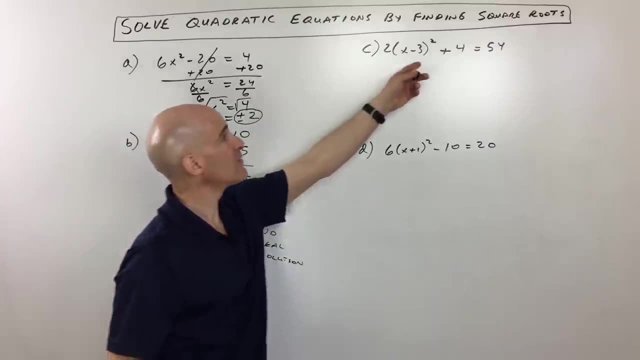 say that there's no real solution. Okay, It's an imaginary solution, So we'll just say no real solution. So when you take the square root of a negative number- Okay, Letter C, now a little bit more challenging here- We've got two times the quantity X minus three. squared plus four equals 54.. And 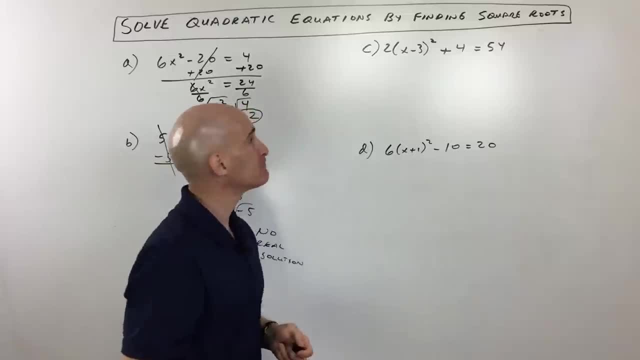 again, what you want to do is you want to work from the outside in towards that X, right? So what I'm going to do is I'm going to subtract four. That's the kind of the furthest out, so to speak. Okay, 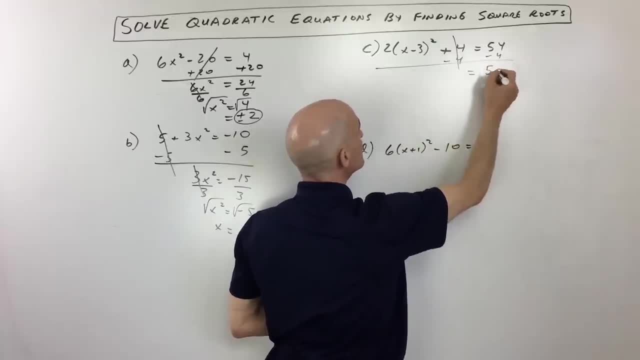 Furthest away, And so that's going to cancel and that's going to give us 50.. And then over here we have two times X minus three squared. We want to then divide both sides by two. Okay, So you can see how we're narrowing. 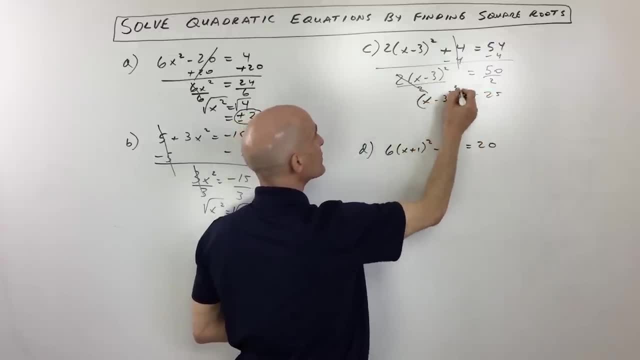 Narrowing down, getting closer to this X. Then we want to say, well, what's the opposite of squaring? We want a square root, Okay. So we want to get rid of that square there. So square roots, that's going to be: X minus three equals plus or minus five. Now, this is a lot of students miss. 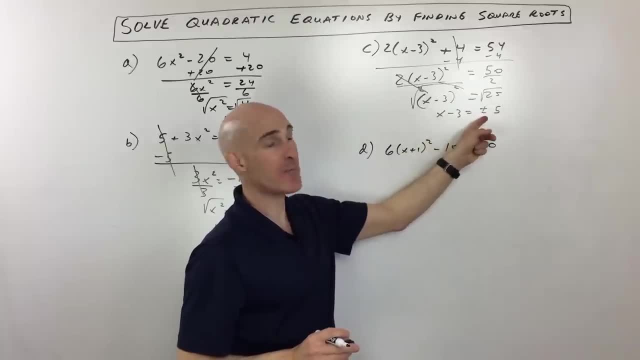 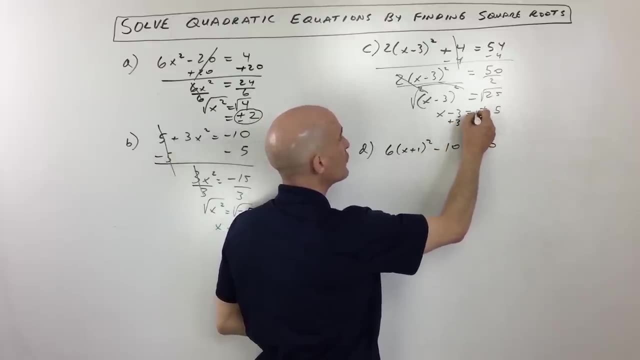 this point here, because as soon as you take the square root, that's when you want to add that plus or minus sign right. And then the last step, also a little bit confusing for some students: you want to add three to both sides, but put that plus three in front of her, to the left of that plus or 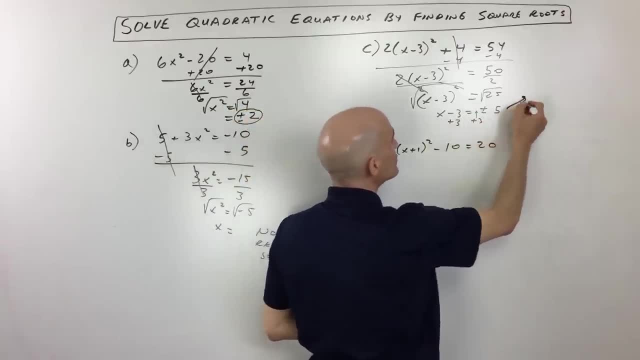 minus sign. That's important. The other way to do this Problem. Okay, A lot of students will do it this way. I think this is a good technique. Split this up into two equations: X minus three equals positive five. X minus three equals negative five. 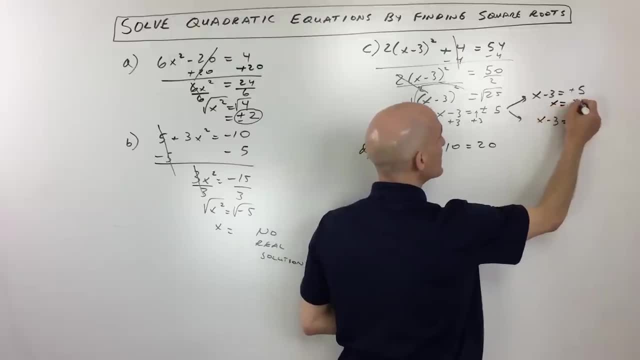 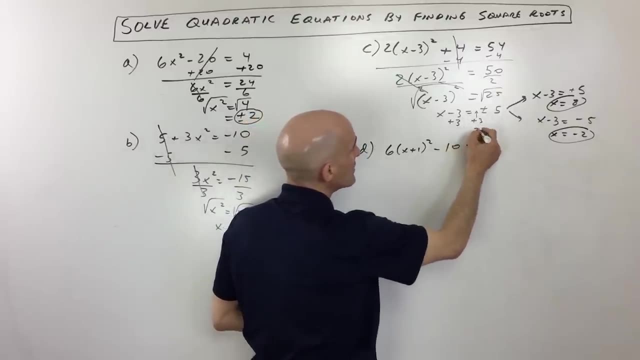 and then solve those individually. So you can add three, That's going to give you eight, And if you add three here, that's going to give you negative two. But if you like this method, you just put that plus three in front, So that's going to be three plus or minus five. three plus five is eight. three minus five is negative two. 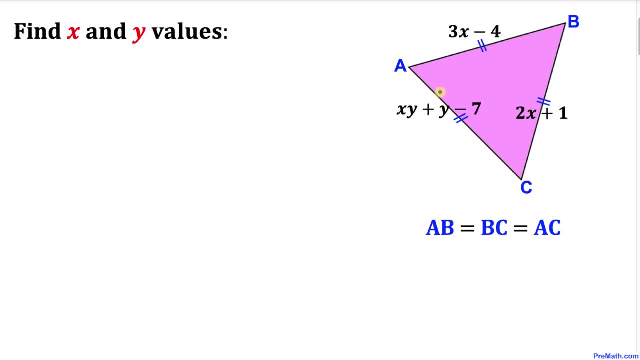 welcome to pre-math. in this video tutorial we have got this equilateral triangle, a, b, c, as you can see in this figure. in other words, a- b- this side length a. b equal to this side length b. c equal to this side length a- c. and now we are going to calculate the x and y values. so let's.